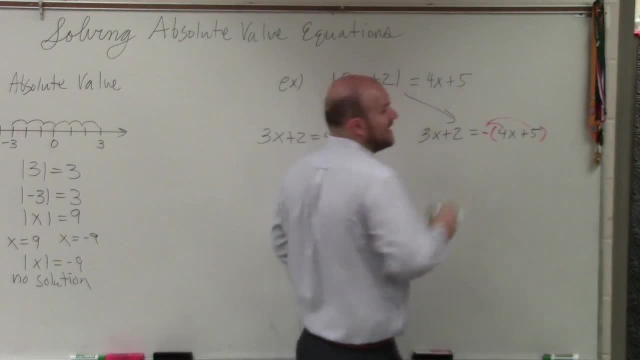 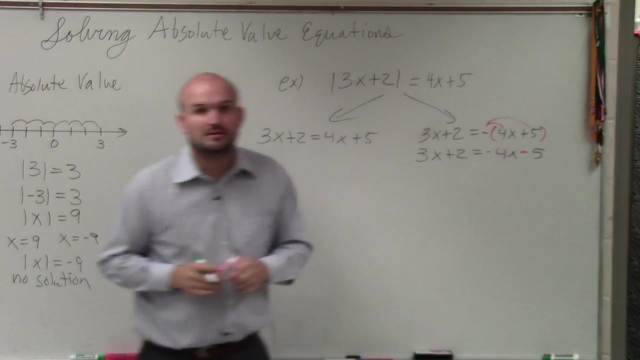 negative outside of the parentheses. Just to remind myself, I have to apply distributive property and basically negate both of them. So really this looks like 3x plus 2 equals negative 4x minus 5.. Does everybody see that? So now we just go through that and go ahead. 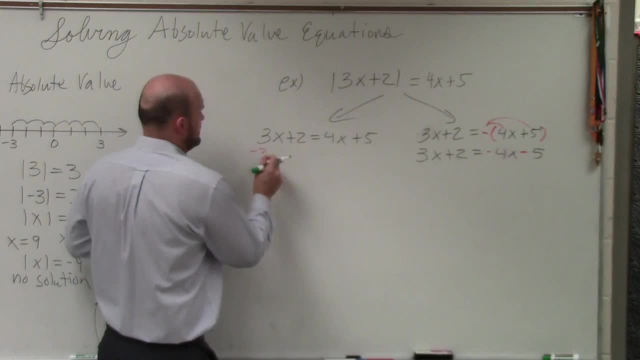 and solve Again. we want to solve for a variable where it's going to be positive. So I'll subtract the 3x, subtract the 3x, I get 2 equals x plus 5.. Subtract 5, subtract 5. Negative. 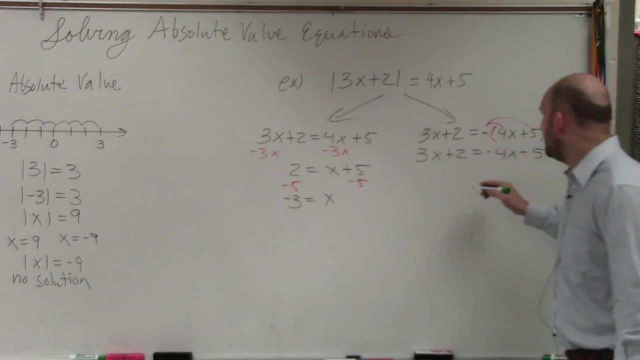 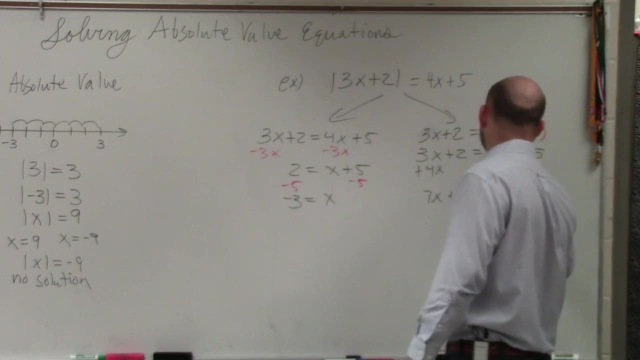 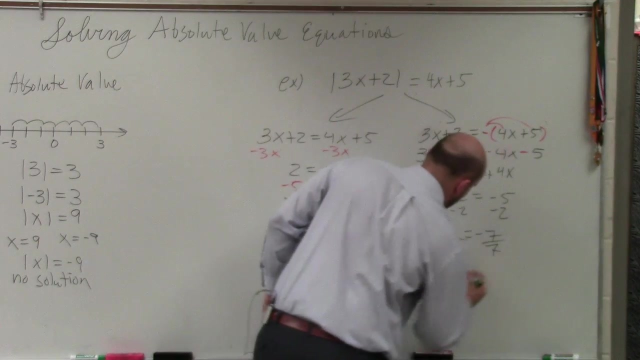 3 equals x. Over here I'm going to add the 4x Onto both sides, So I get 7x plus 2 equals a negative 5.. Subtract 2, subtract 2.. 7x equals negative 7.. Divide by 7, divide by 7.. x equals negative 1.. Does everybody see how? on this, 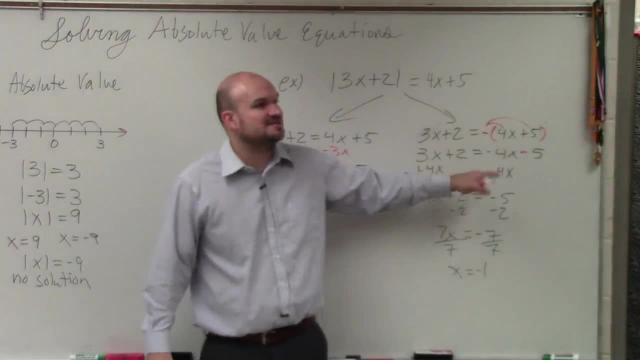 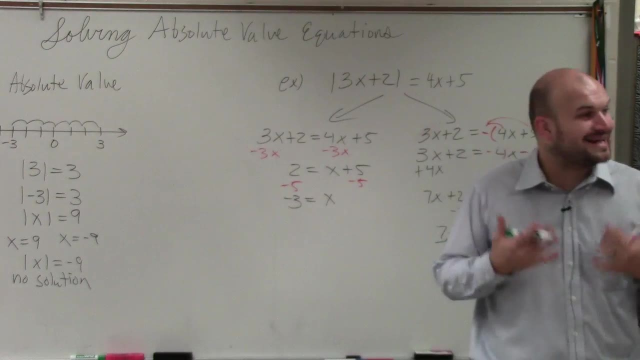 example, it was easier for me to solve for x on the right-hand side. And this example was easier for me to solve for x on the left-hand side. Again, guys, you don't have to follow the way I do it, But just through my years of experience, I like solving. I like solving. 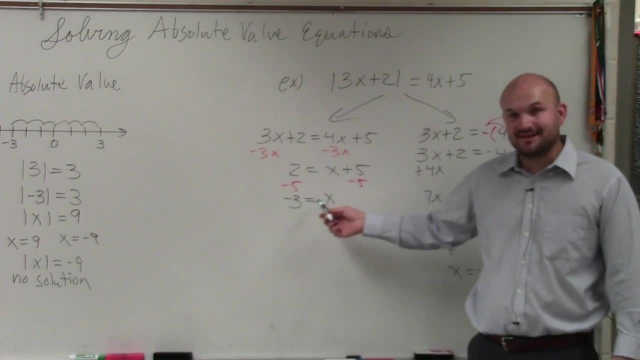 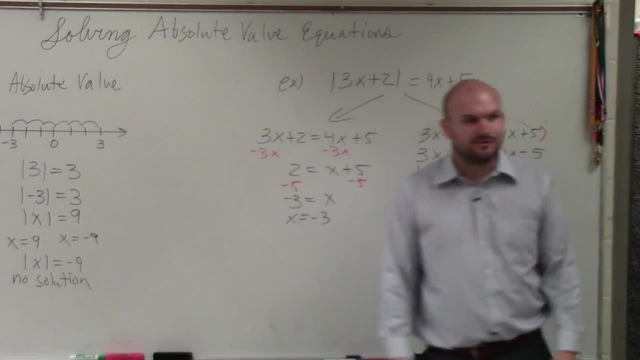 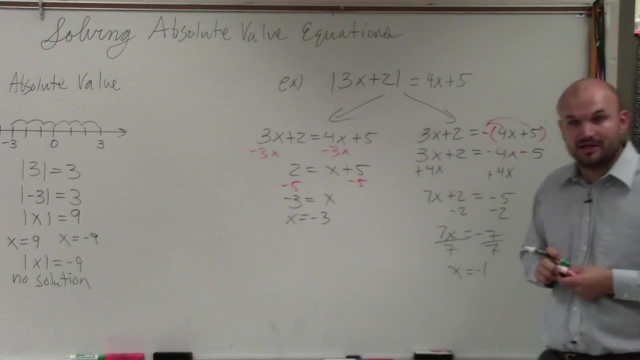 just switch it. We're allowed to do that. Just switch it. Switch it back over after you've solved. Now we need to go back and plug it in. Now I can tell you guys, you can plug in x, You're. 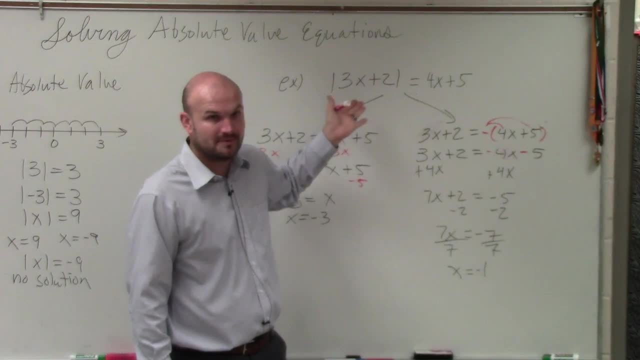 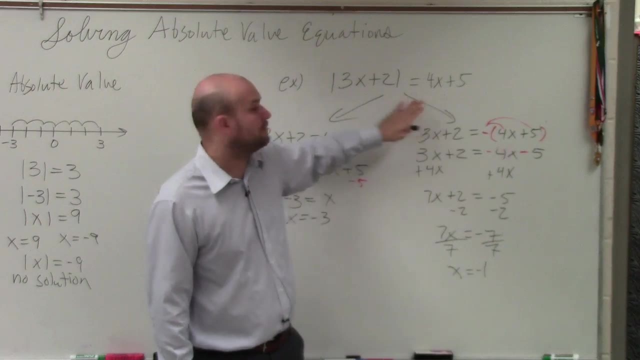 supposed to plug in x for the x's on the left-hand and the right-hand side right, But I think the easiest thing for me, the easiest thing to do, is just plug it in on the right-hand side, Plug it into the equation where your absolute value is equal, because what the absolute 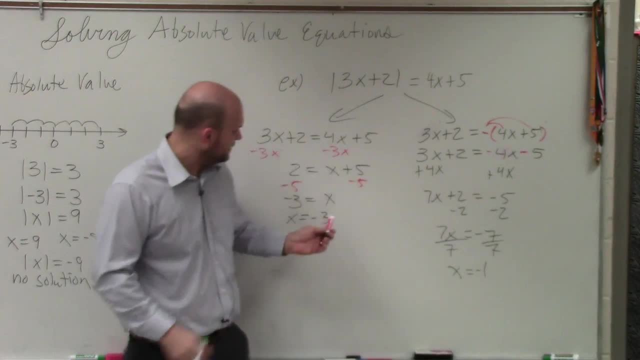 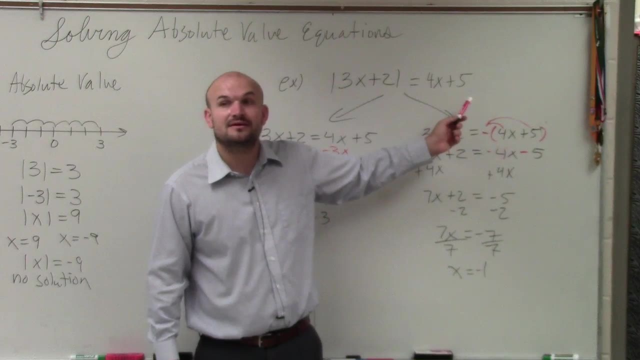 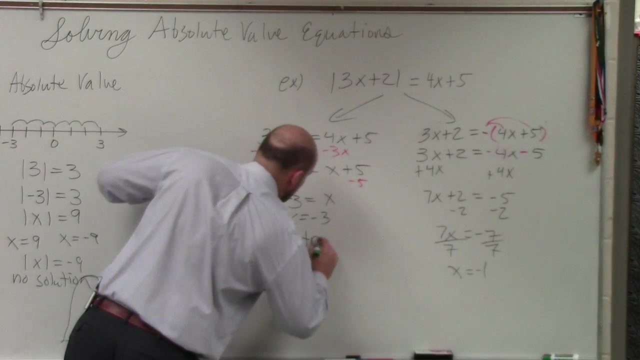 value is equal to has to be a positive number. So watch When I plug in negative 3 on the right-hand side, 4 times negative. 3 is negative, 12 plus 5 is negative 7.. Can the absolute value equal a negative 7? No, So this is extraneous. Now let's try negative 1.. When you plug